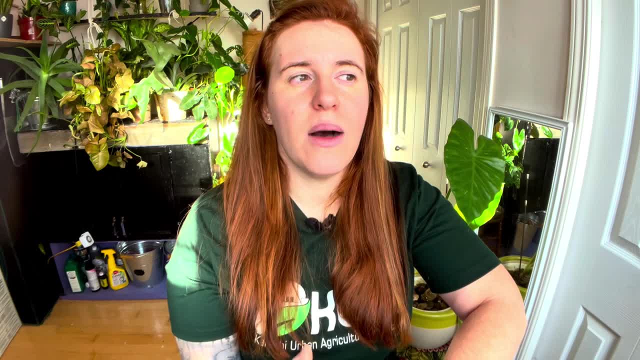 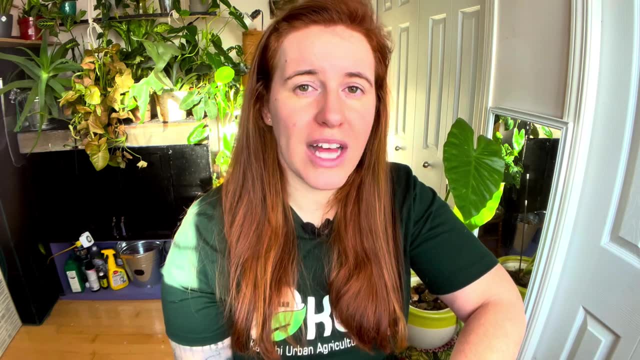 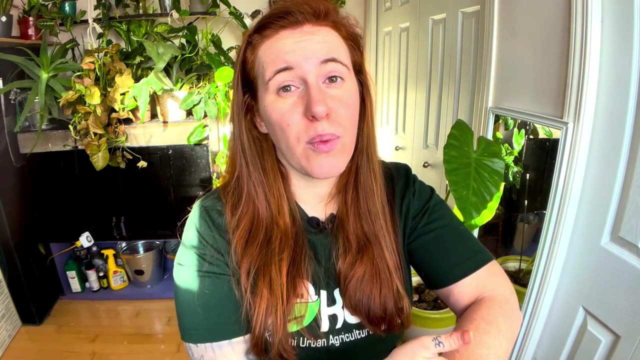 it that way, the fact that hydrogen and oxygen are macronutrient. I would implore you to quite honestly look at how much you let your plants dry out between waterings. Now that you know that these nutrients are considered essential for plant survival, will you change the way you choose to? 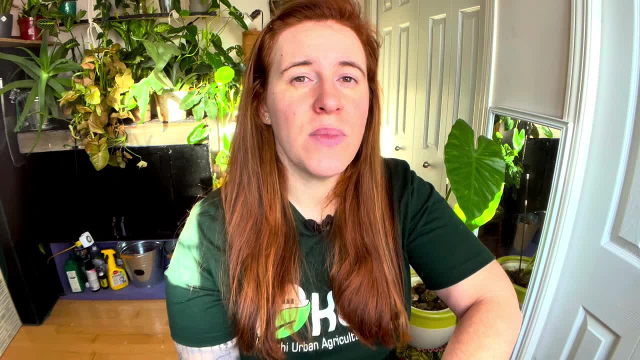 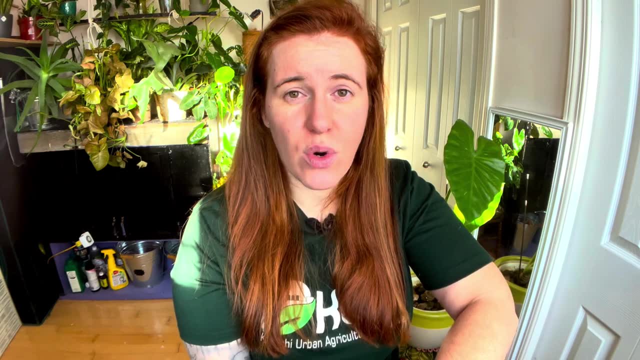 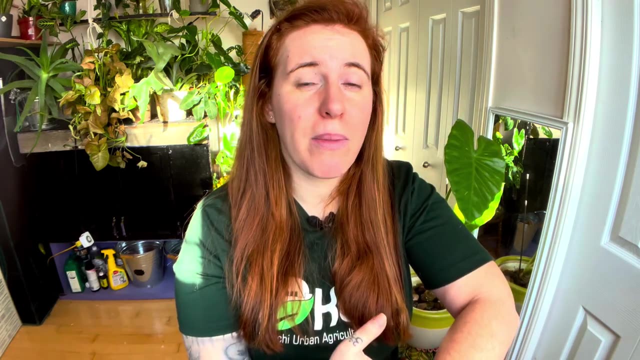 water your house Plants or your indoor plants in general. I encourage you to go with a more porous medium that allows for more air exchange or air infiltration to help with the microbes and support aerobic microbes rather than anaerobic microbes, But I also encourage you to keep that. 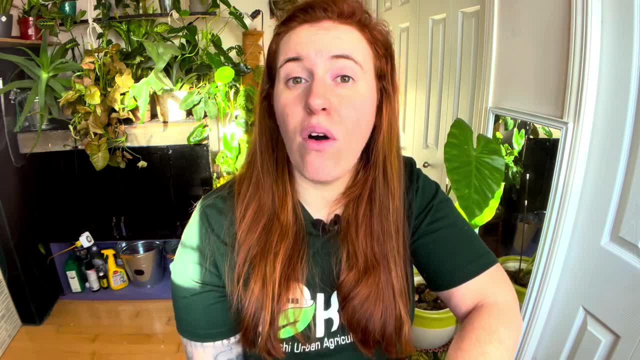 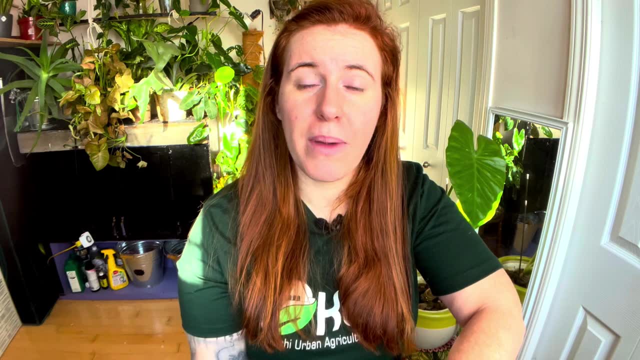 soil moist- relatively moist- at all times, And so long as you have the air that you need present to support aerobic rather than anaerobic microbes, you will be just fine. you will not get root rot. root rot does not happen in the presence of oxygen. 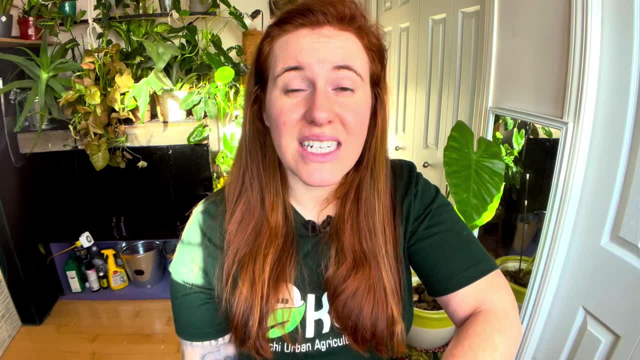 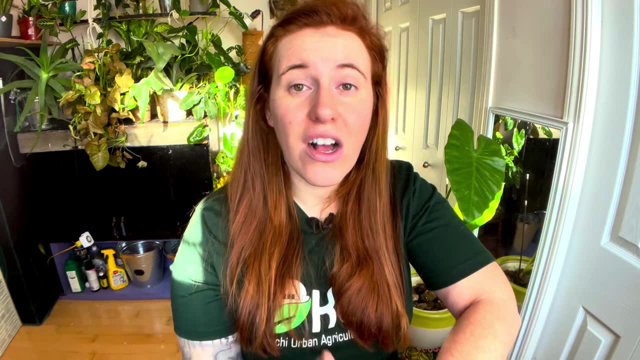 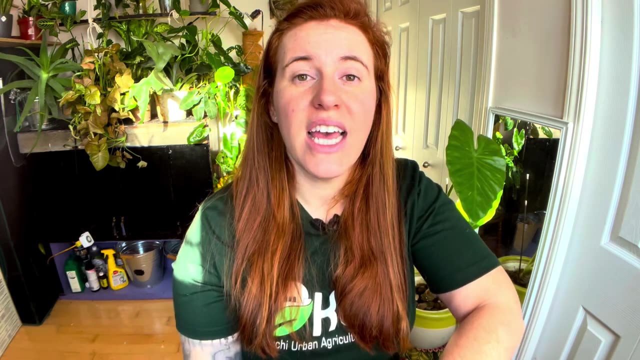 But damage to the plant, yellowing leaves, stunted growth. that sort of thing does happen when we don't have enough hydrogen And we don't have enough oxygen, we don't have enough essential nutrients And, for all intents a purposes, a huge portion of that nutrient is taken up in a soil. 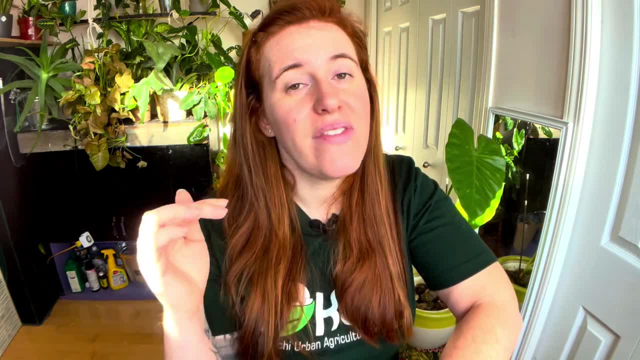 solution, meaning a slurry of some sort that needs the presence of oxygen If your soil is cancerous or not stuff. So you want to be tracing about how easy it is to brasile or adapt your plants as soon as possible. You're taking is araz to green einfachtwo. 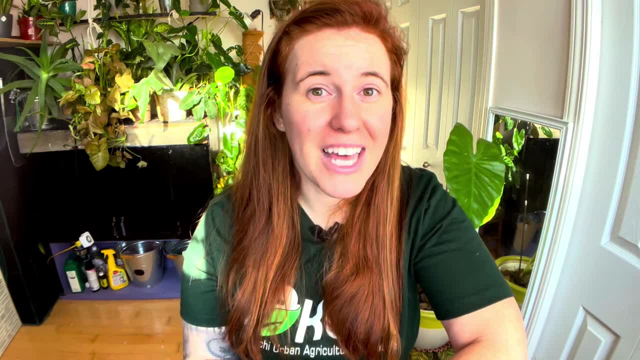 and we're going to wash our plants. You're taking this into general care. to shell themarraz, everyone floor in our backyard orよ of two hydrogens and an oxygen, something we like to call water- h2o- to be present. so you are starving. 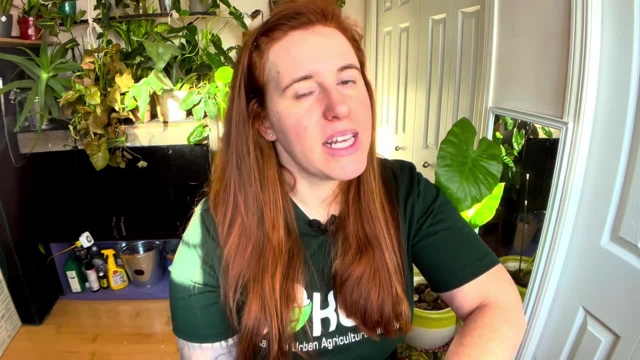 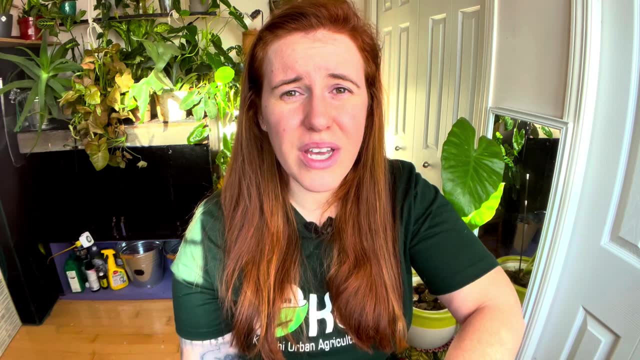 your plant when these things are not around. so just keep that in mind. how long could you go without food and water? you know, water i i don't. i think it's like two or three days, not even that you could survive. that's if you're like sitting still and doing nothing food, you can go a little. 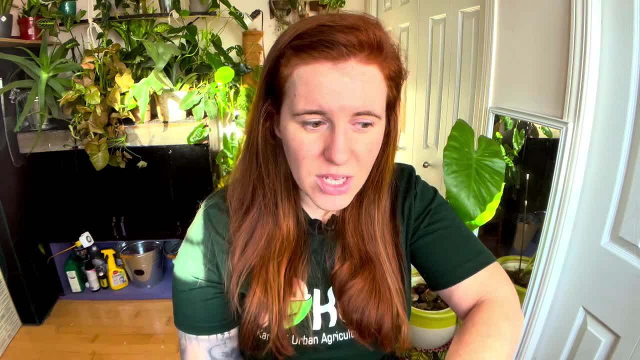 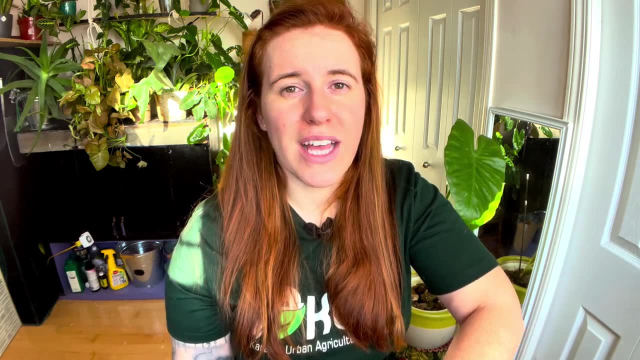 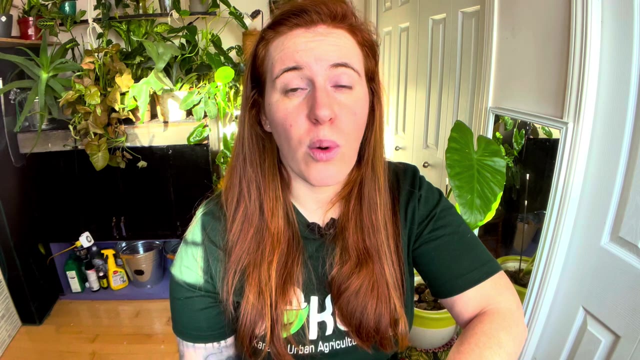 bit longer, but water you. you really do need that in plant. you know work on the same spectrum. now, of course, there are oddities to this. there's going to be your c4 plants, which we talked about in our sansevieria sansevieria video, where we talked about snake plants potentially being c4. plants and how they have different mechanisms in which they can support themselves in the absence of water, and things like succulent and cacti also fall fall into that category. but just keep in mind the rest of your plants, don't? they are c3 plants and they do need water in some at some point, and 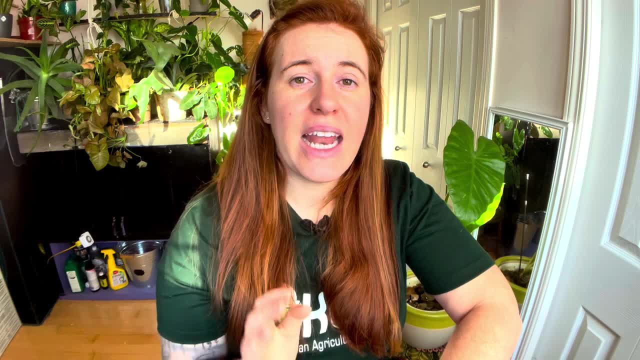 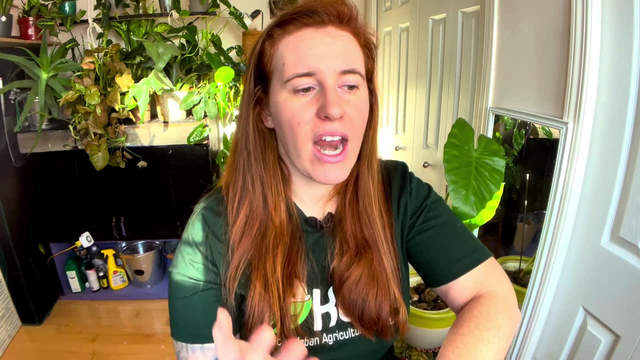 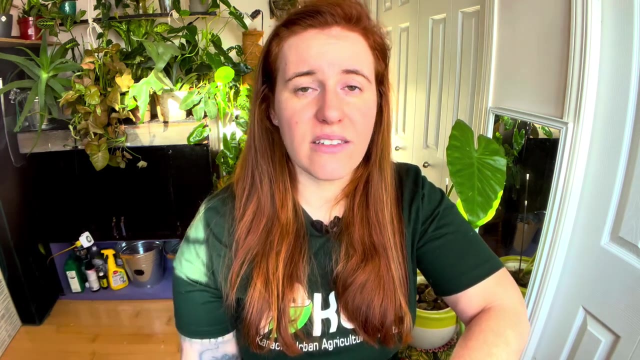 at on it can a relatively continual basis. so now one thing with hydrogen that i do want to drive home, because there isn't a ton to talk about when it comes to hydrogen. it obviously comes in the form of water, it's up, taken through mass flow, it's a primary macro nutrient and clearly it functions as a 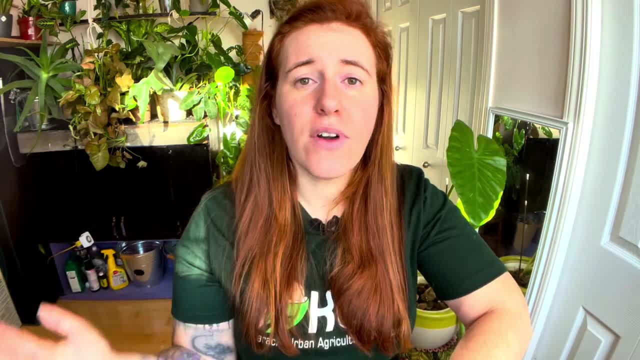 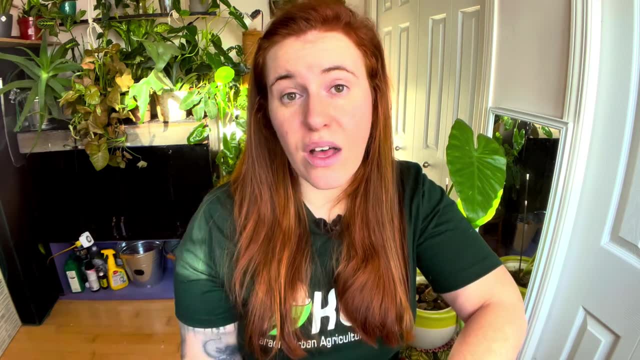 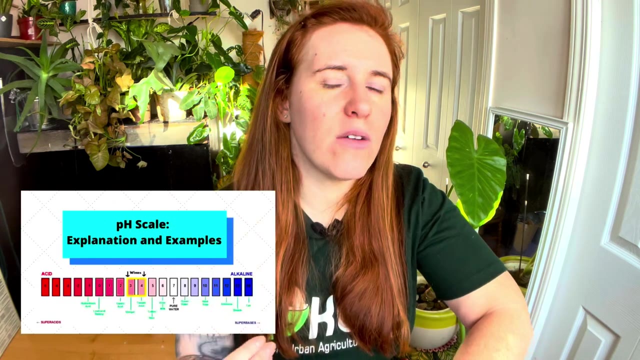 stepping ladder for nutrient to kind of hop its way up from the soil to the root and etc. through the entire plant. and another really important factor of hydrogen to the plant as a whole actually is what in the soil. so hydrogen is what we're counting when we're counting the number of or when we're 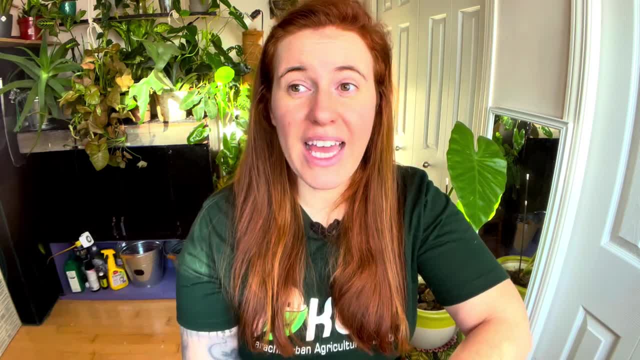 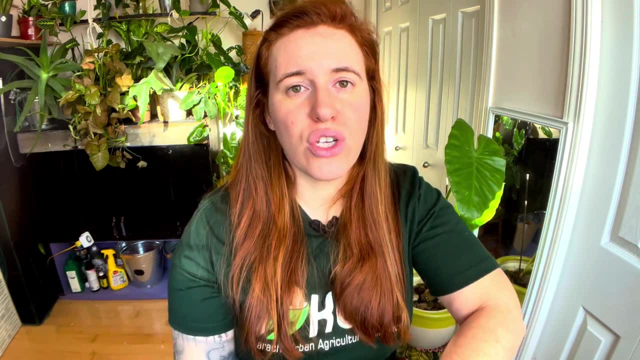 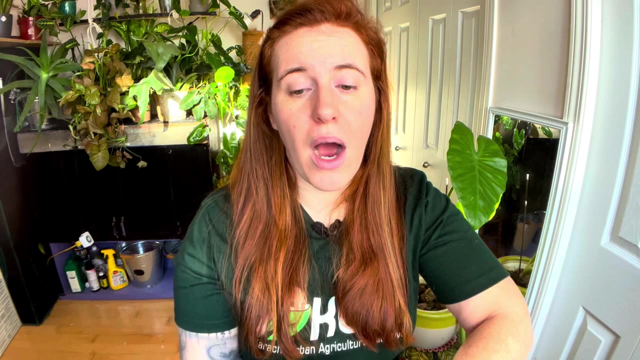 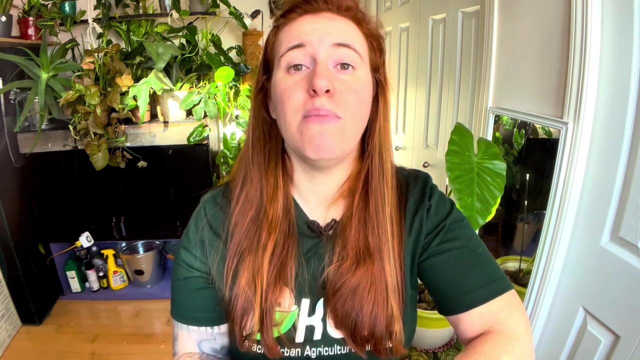 determining the ph. so what we're doing is we're actually counting the total number of hydrogen within our soil solution. so if you remember back to our video that we did on nitrogen, we talked about the potential of gaining or losing hydrogens from our nitrogen molecule. so the forms of nitrogen molecules we had was ammonia and ammonium, so both of which have 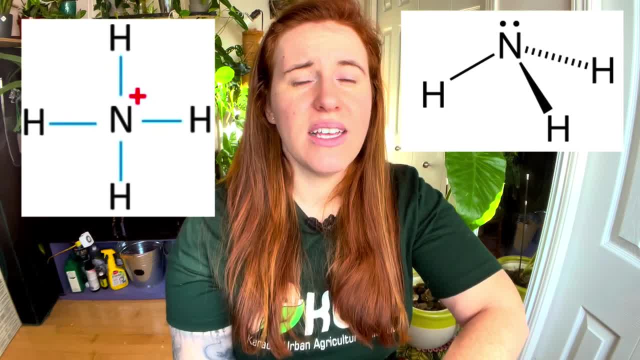 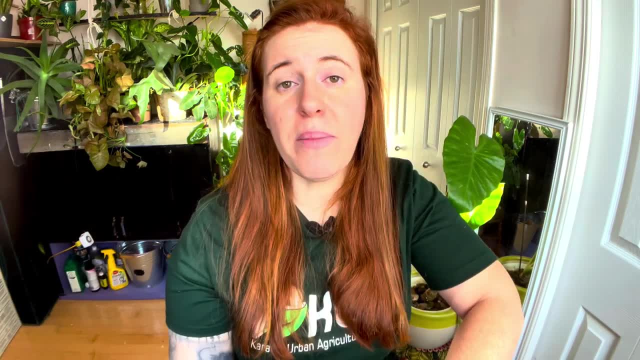 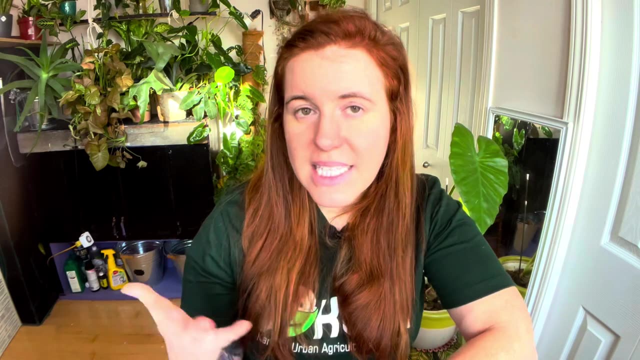 hydrogens attached to them. now we also have molecules such as nitrate and nitrite that can pick up hydrogens and form an even bigger molecule, or in some cases they may lose a hydrogen from that bigger molecule and release it back into the soil so as more hydrogens are released into. 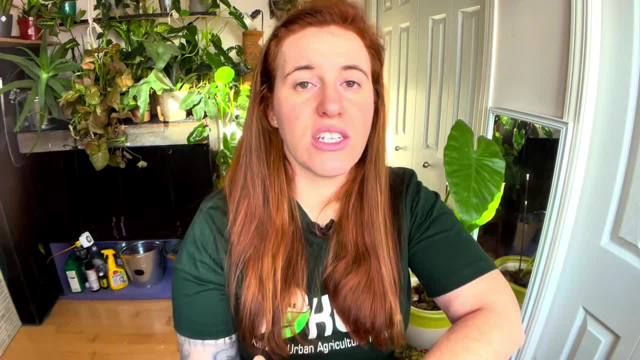 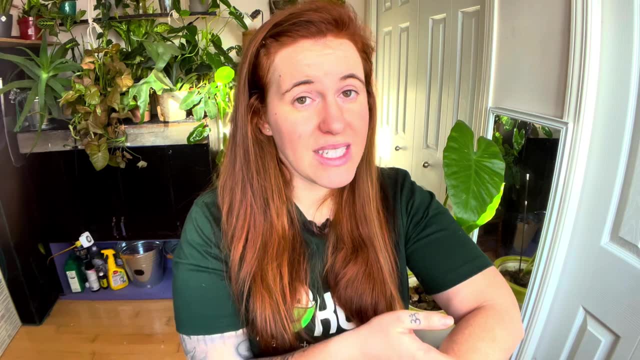 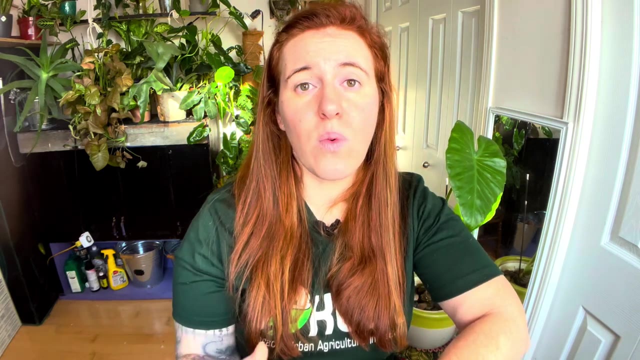 the soil solution and popping off of our nutrients, such as ammonium, for example, we end up with a more acidic soil. the more hydrogens, the more acidic. however, when we reduce the number of hydrogens in our soil, hydrogen ions in our soil, we end up with a more alkaline soil or a more 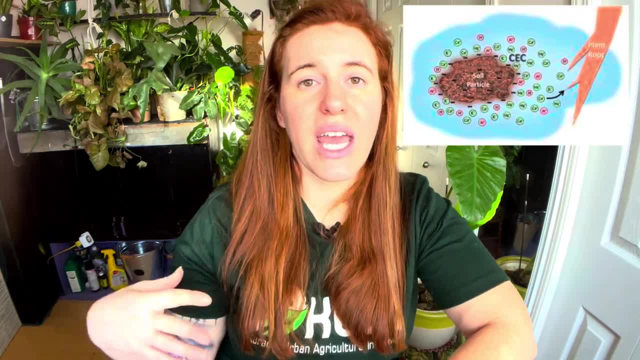 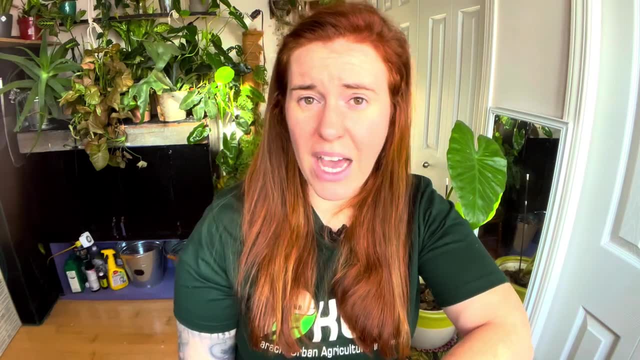 basic soil, as some people like to call it. so we end up pushing above seven on the ph scale. now you're probably wondering: well, how do i add more hydrogen, how do i take out more hydrogen? and this is what we're doing when we're using things like soil sulfur, or we're using 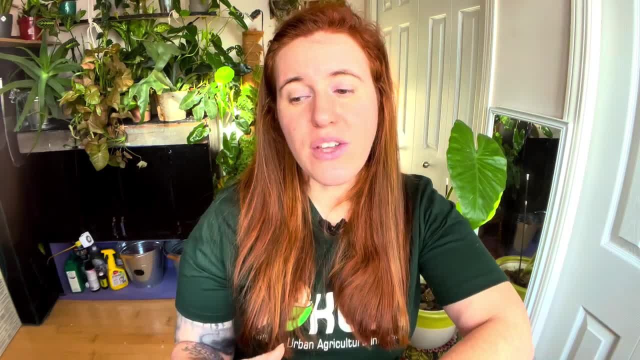 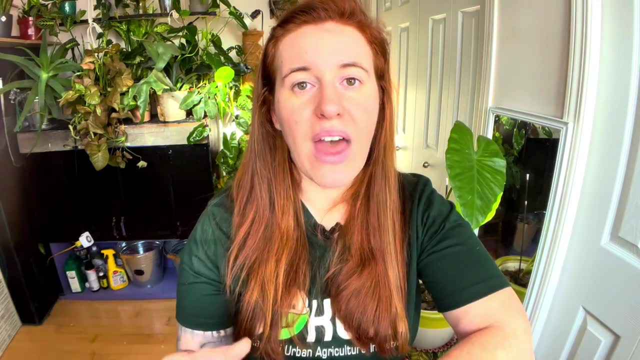 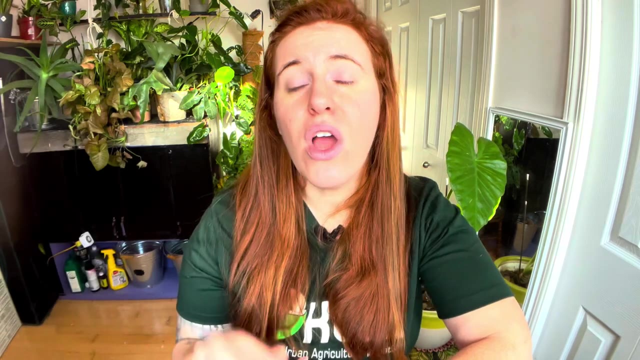 lime, gypsum, that sort of thing. so if we're trying to make a more alkaline soil or we're trying to reduce the number of hydrogens in our soil, we add in components that will bind to hydrogen, so we're not simply just plucking the hydrogen out and vaporizing them into the air. 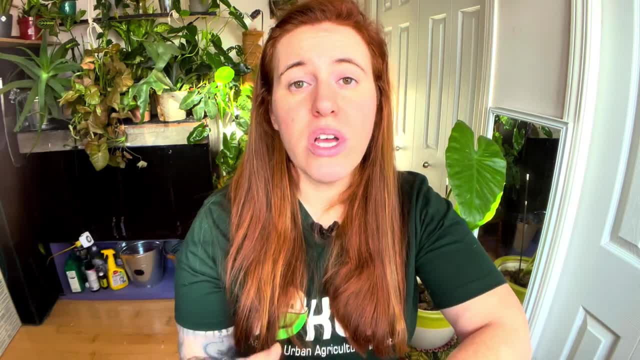 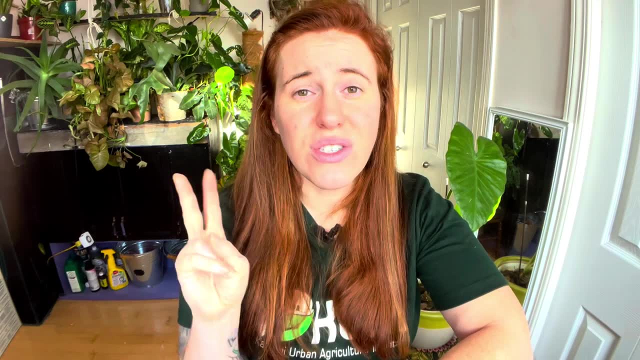 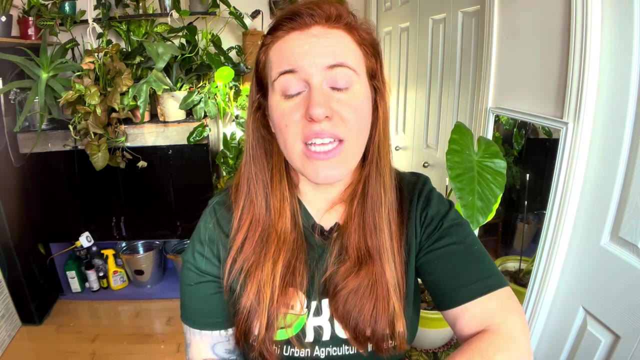 rather, we're binding them to another molecule so that the plant can uptake them and they're not left in suspension of that soil solution in the soil smoothie, as we'd like to call it. so once it's removed from the soil smoothie, then what ends up happening is our ph ends up, you know. 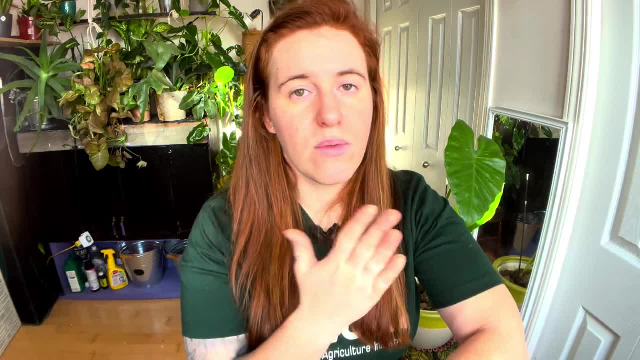 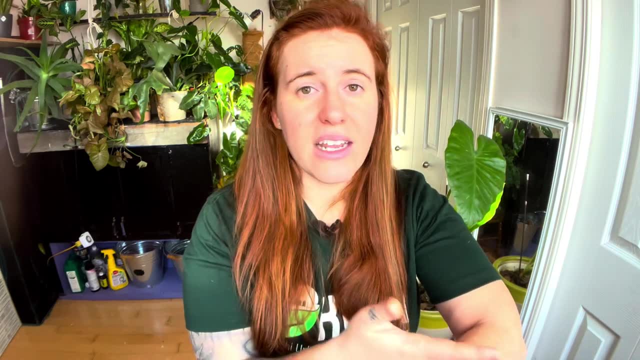 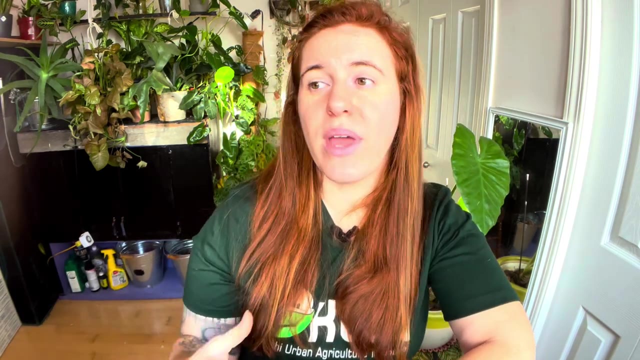 increasing over time. so if we're on, you know, a really toxic range of acidity, say a ph of four or you know five, then when we add things that help increase that, we're actually pulling hydrogens out of solution. conversely, if we have a very alkaline scenario- say we're have a ph of eight- 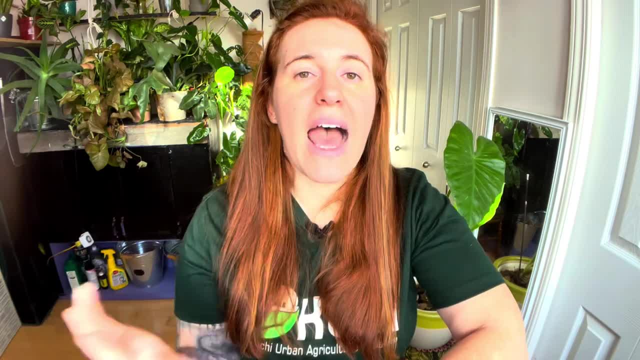 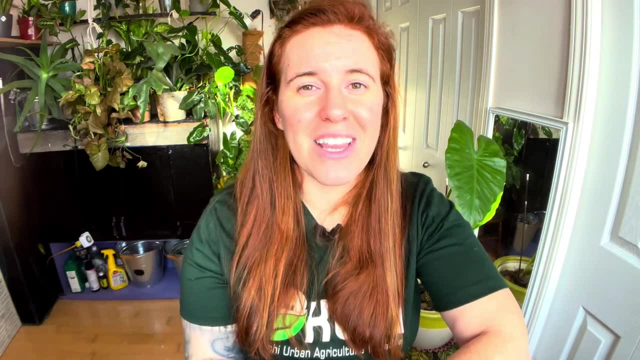 or nine and we're trying to bring it back down. we're actually pulling hydrogen out of solution. we need to add hydrogens to the soil solution. so this um for hydroponic growers comes in the form of a little bottle, and the little bottle you put drops in and all that's doing is it simply. 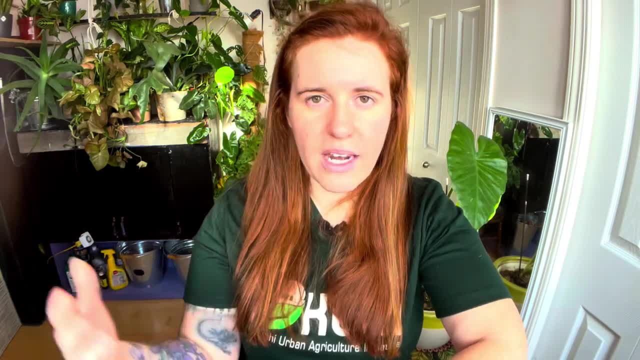 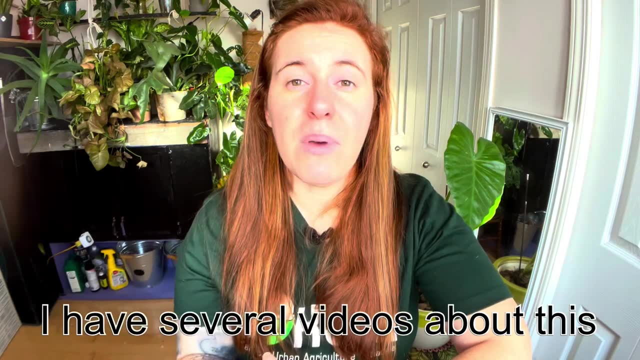 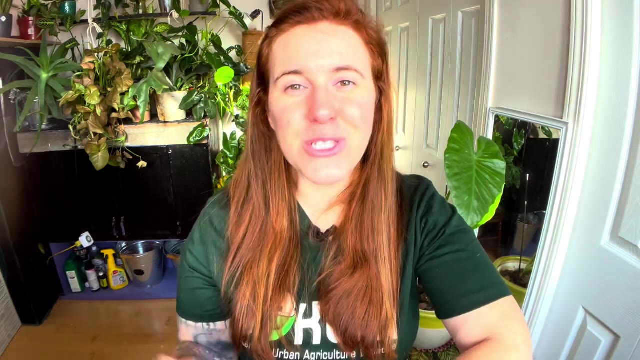 adding, adding hydrogen molecules to the solution or again removing them. but for us plant people to change that ph again, we have to have additions. now keep in mind, there's a wide range of different plants out there, all of which kind of have a different preference for how many hydrogens they. 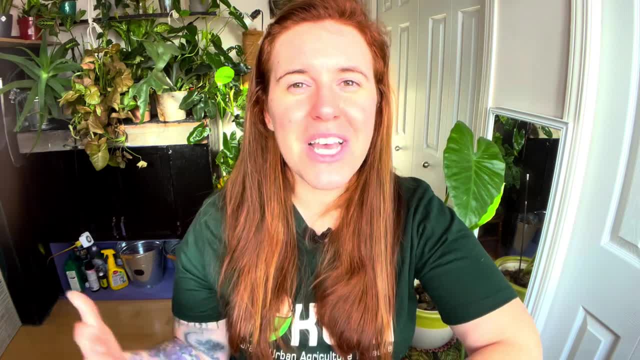 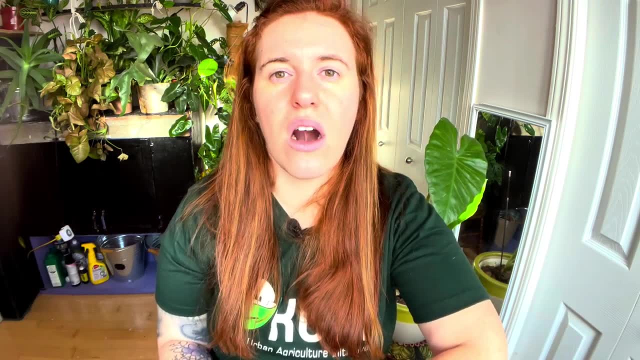 need to survive in and what you need to thrive and survive in. so always make sure you look up what your particular plant enjoys most and then adjust according to that. but that is all i have for hydrogen today and i hope you guys enjoyed. if you did, be sure to give this video a thumbs up. 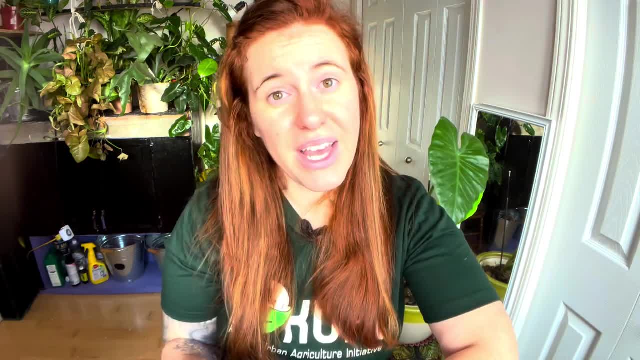 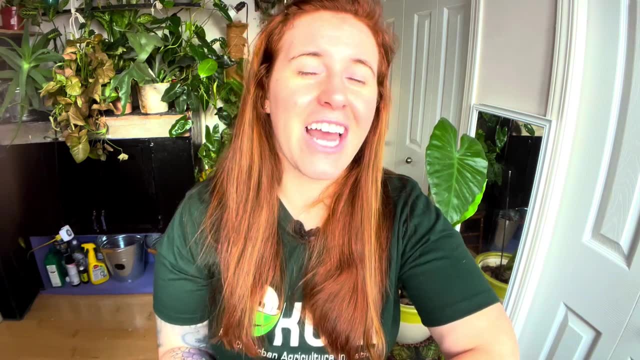 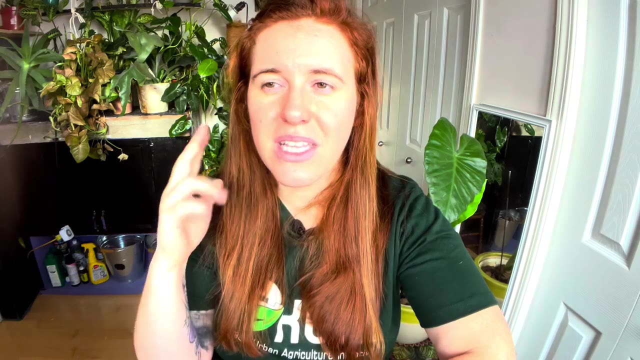 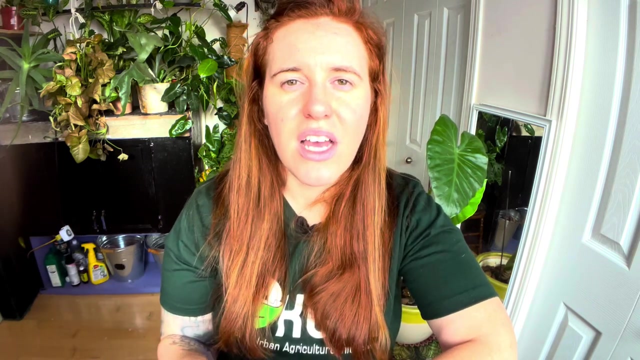 and i'll see you in the next one. bye, bye up. let me know in the comments down below what you learned new in this video. it just gives me a little bit of an idea as to where you guys are at in both your soil and your plant science knowledge. 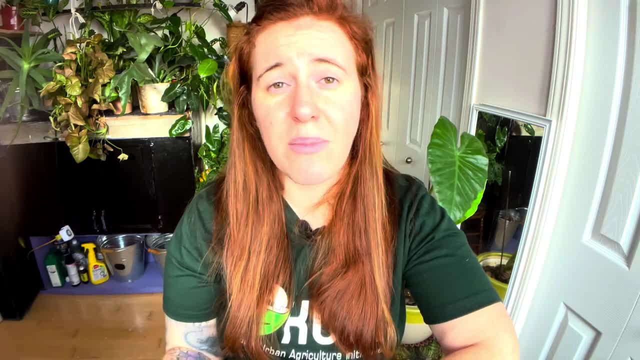 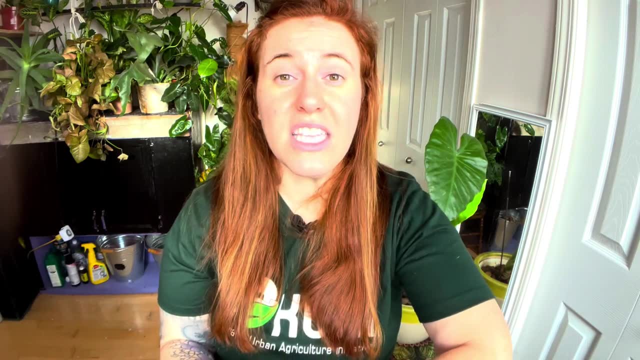 i'm not, you know, offended if you know nothing and i'm not offended if you knew everything. quite honestly, it's just to give me a bit of a feel, to gauge what type of videos you guys want in the future. but anyways, i want to thank you guys for- and the reason i say that is because some of